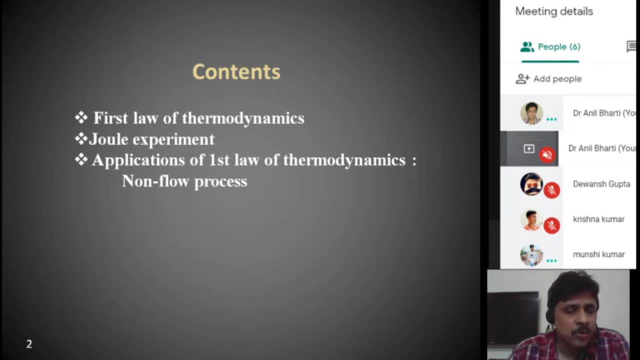 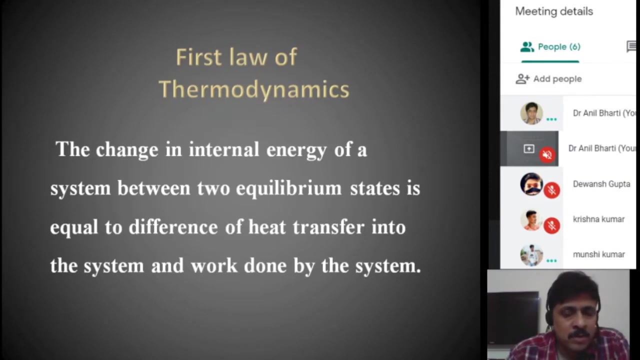 This law is also known by non-flow processes. So under this first law we will study constant pressure process, constant volume process, Then constant temperature process, if we got enough time, And then we will discuss a few numericals or some illustrations. So first start with the definitions of first law. 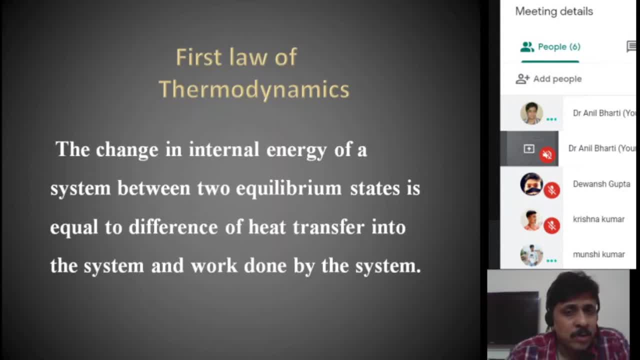 Now, according to various- you can say- studies, they have shown that the first law is the change in internal energy of a system between two equilibrium states. Now, what does it mean? Whenever the system undergoes shifts from one state to another state and we consider that both the states are in equilibrium, are equilibrium states. 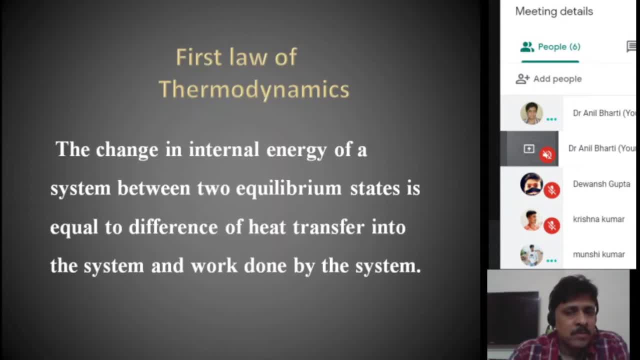 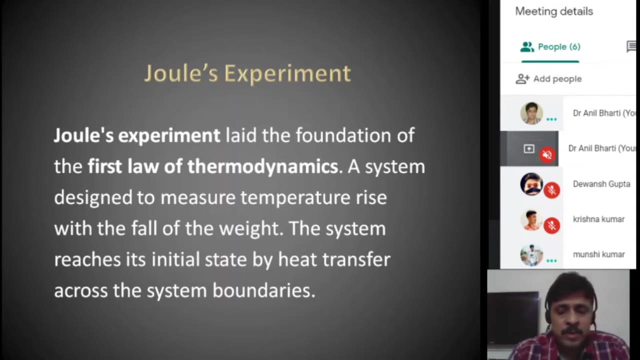 Then the total amount of energy interaction is equal to the difference of heat transfer into the system and work done by the system. Now the first law of thermodynamics is very much, you can say, interesting. There is actually very well very powerful different theories about heat transfer. 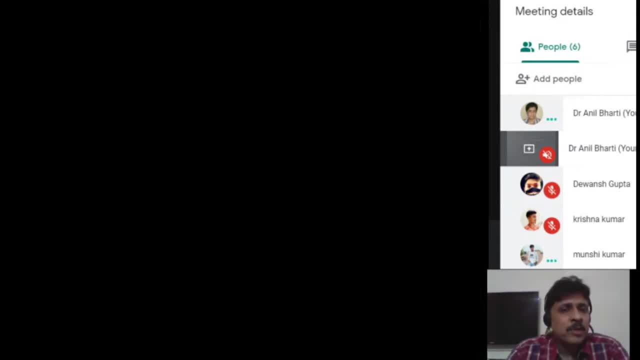 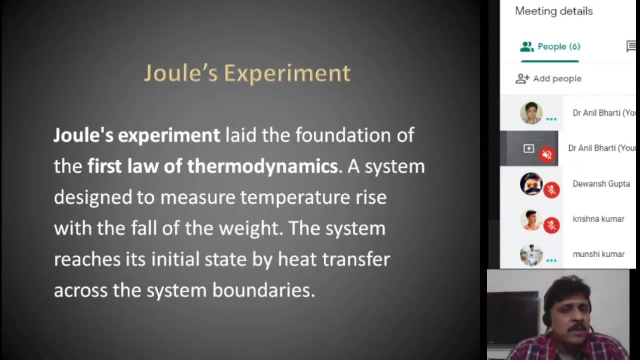 Now, this theory was basically governed by the Joule experiment. Now let us see what is the Joule experiment. So Joule's experiment laid the foundation of the first law of thermodynamics. Our system is designed to measure the temperature rise with the fall of weight. 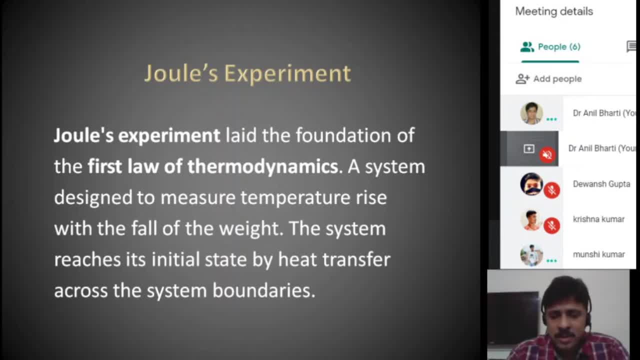 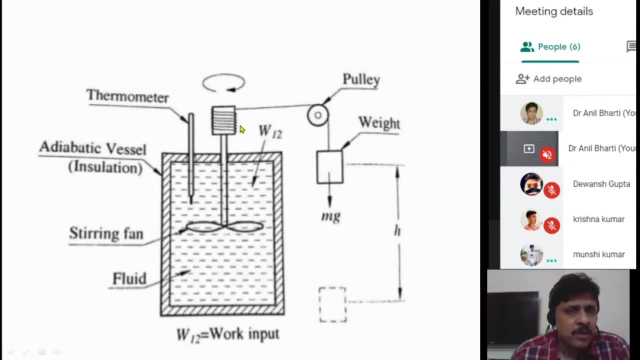 The system reaches its initial state by heat transfer across the system boundaries. Now Joule had designed an apparatus, very simple apparatus, in which he tried to, you can say, translate between complicated conditions, translate the work into the heat. This is a pulley, and he wound up the few threads on. 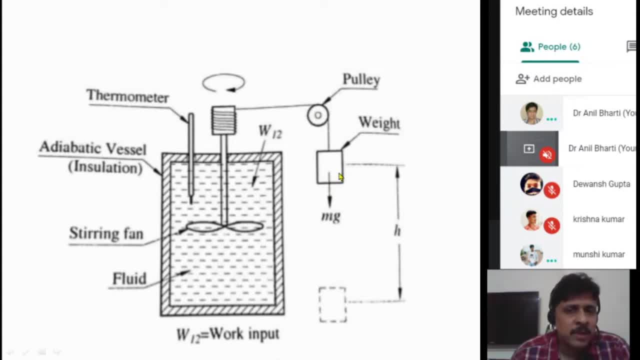 this pulley and on the other side he suspended some known amount of weight. Now, can you judge what will happen when he will keep this weight to fall free from this height? What will happen in return? this, it will try to revolve this fan. Now we can easily calculate the amount. 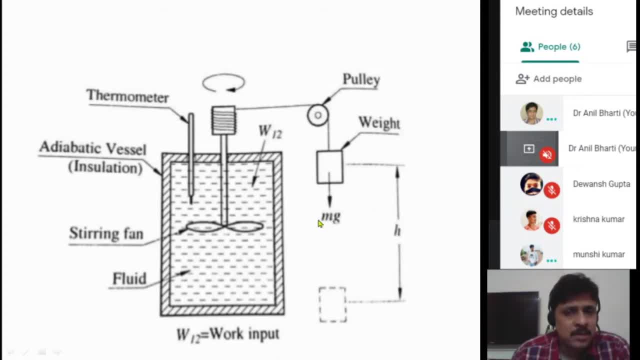 of work done by you can say mgh. It should be equal to the heat energy translated into the system. Now, how will the heat energy come from here? Now, heat energy is generated due to the churning of water inside this system. Now, when this fan revolves, when it rotates, what will it? 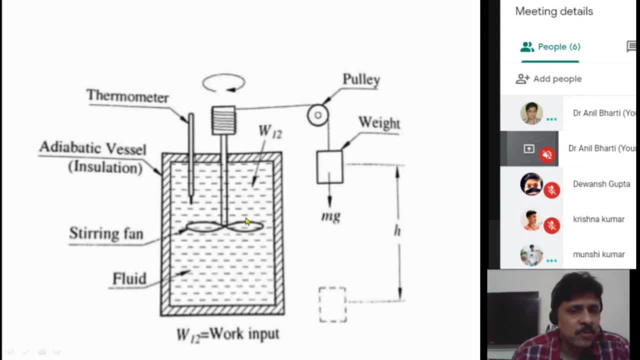 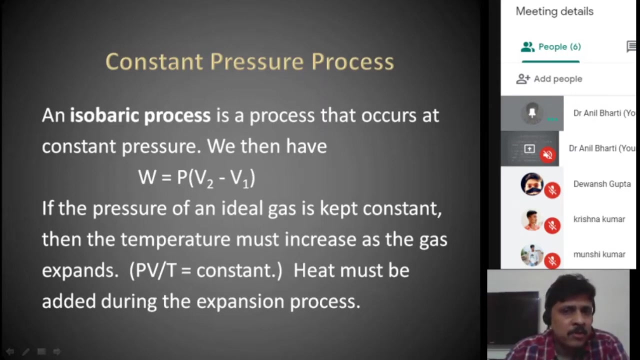 do, it will churn the water and because of that you can say very small amount of heat is produced or temperature is raised in the system. So in this way he tried to calculate the. Now what is the effect of work done on the system? Constant pressure process is also known as isobaric process, in which the process in this 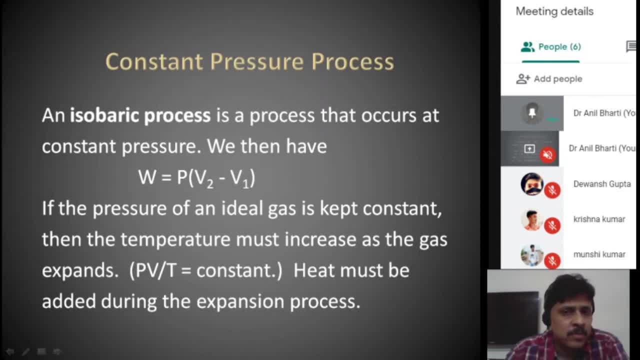 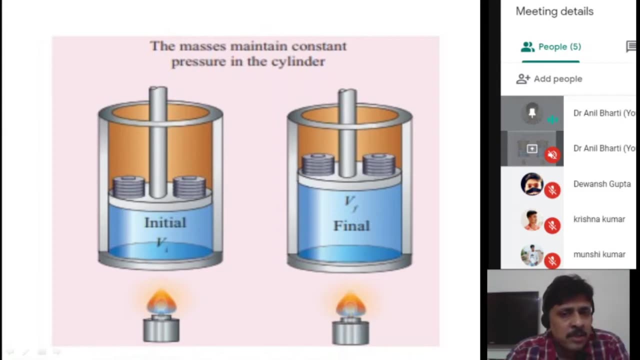 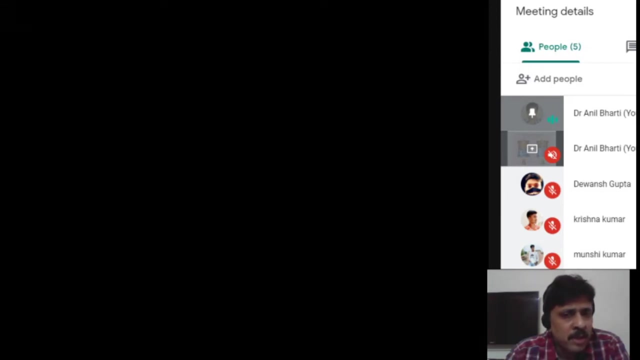 process. the pressure remains constant throughout the process. So then we can say that W is equal to pressure multiplied by V2 minus V1.. This process like this, let us say there is a piston and cylinder arrangement. Now we put some weight on the piston so that it can put pressure on the gas which is enclosed. 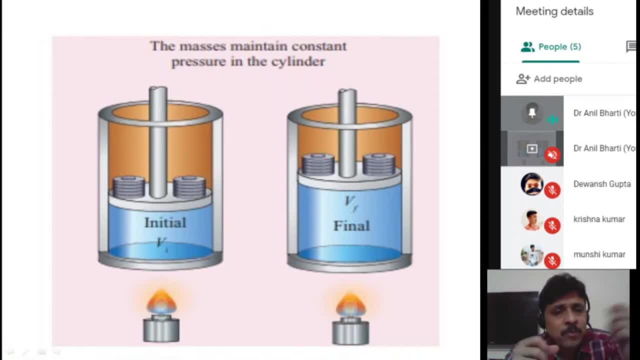 inside the system. Now let us say we want to keep the pressure constant. Just, we intend to keep cylinder. So when the pressure increases the piston will move upwards and in. during this process the pressure will remain constant because whatever the there is in pressure, 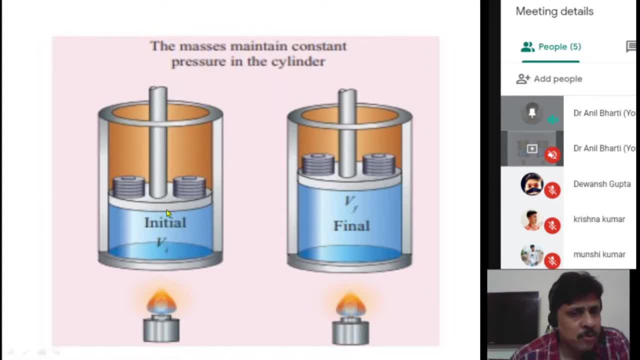 The piston will Proportionally. Proportionally move back and forth in the similar fashion, So like, for example, here we have supply, some amount of heat. This is the initial coordinate: P1, V1 and T1 and this is the final coordinates. Once the heat is supplied into the system, piston moves backwards. 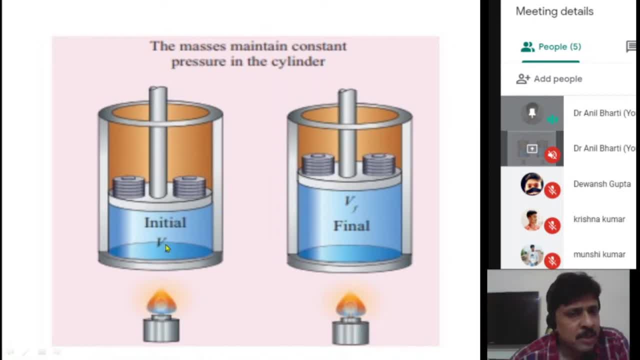 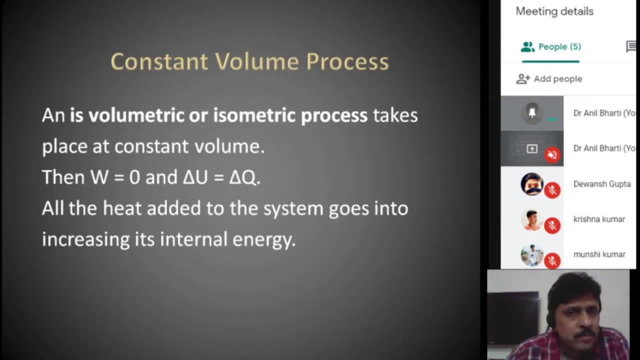 but still the pressure remains constant. So here we can write it as V1 into T1, into V2 into T2, because pressure, temperature and volume is constant, but pressure is Sorry. pressure and temperature, temperature is varying and pressure is constant. So again we can write: 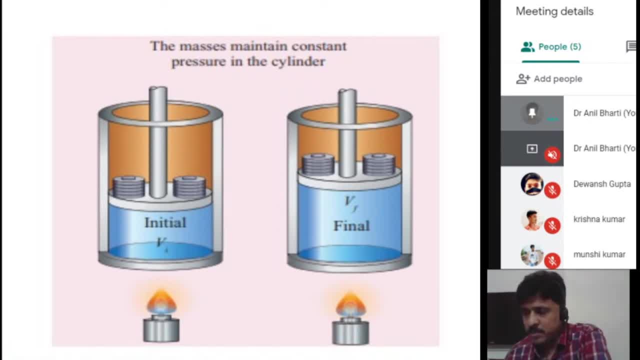 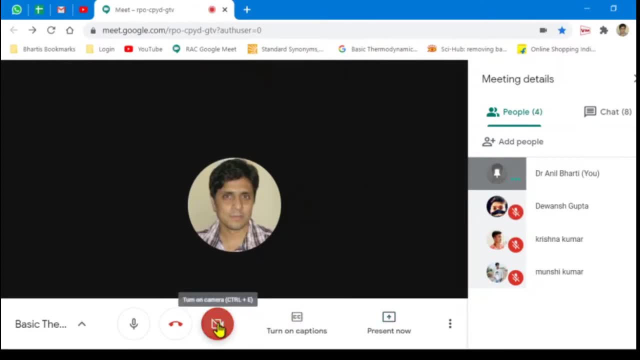 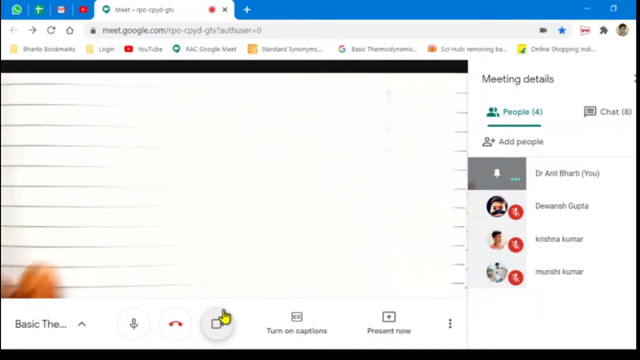 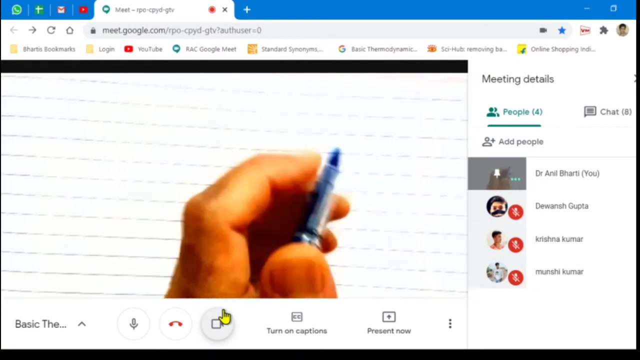 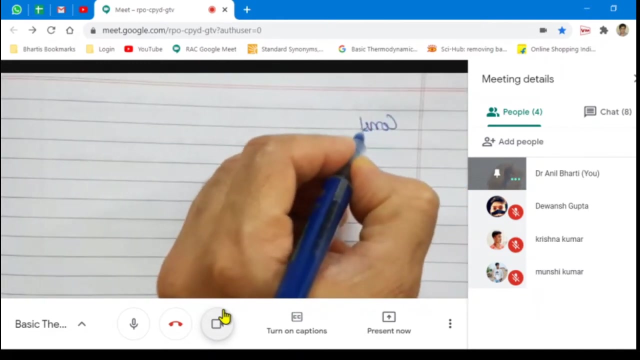 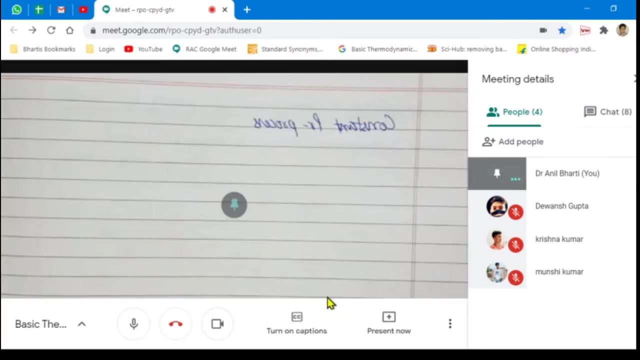 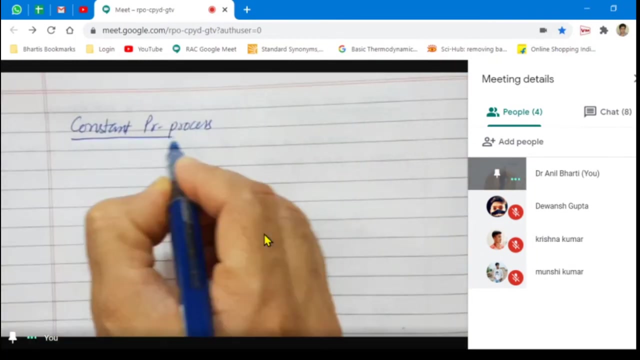 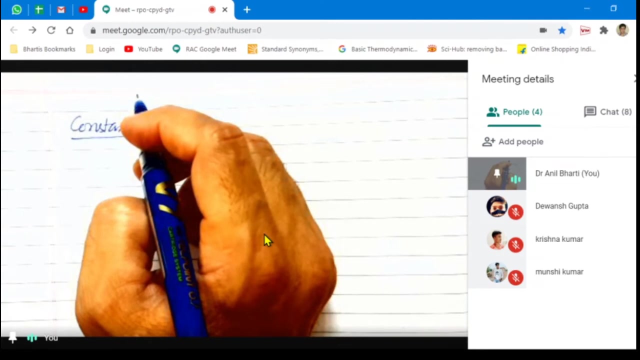 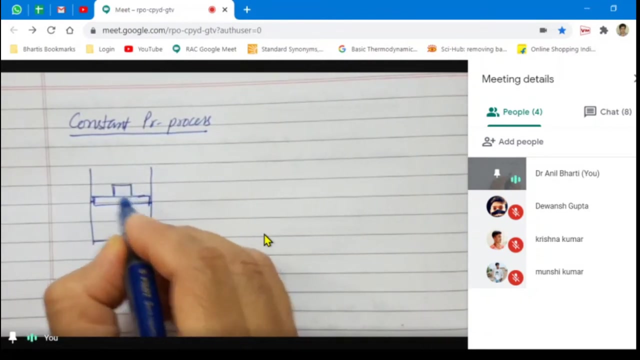 an equation for this. Thank you. Now for a constant pressure. we assume that there is a piston and slender arrangement. We have put some weight on the piston and there is a gas inside this closed system. Now, when we supply some amount of heat here, that is P1,, V1 and T1, since the piston is free. 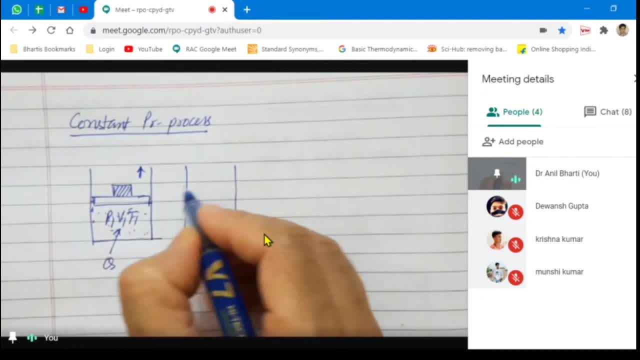 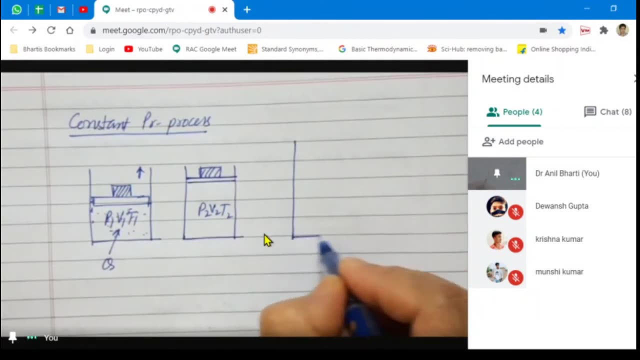 to move. so piston will move in upward direction, so it will change its position just to keep the pressure constant. So here the final coordinates becomes P2, V2 and T2.. So now if we can draw this pressure volume diagram, 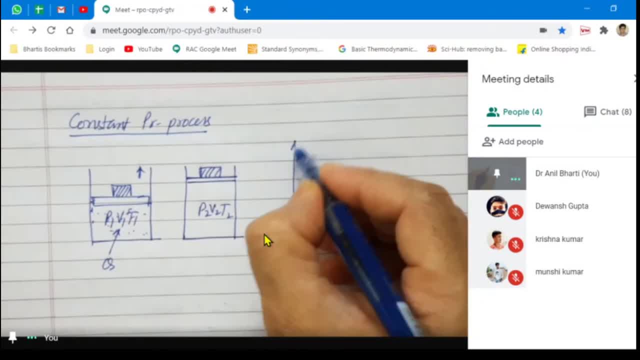 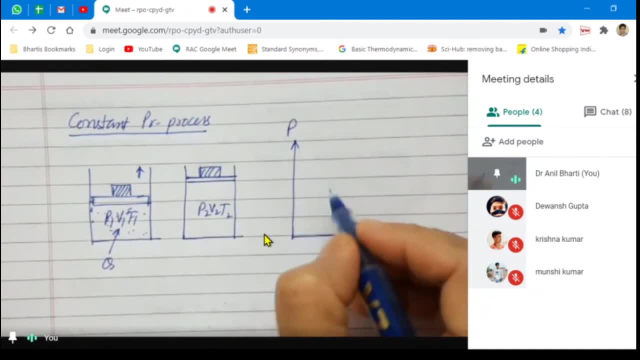 So what will we get Here? you can see that pressure is constant, but volume is changing. So let us say: first there was volume is V1, the coordinates, of system coordinates- were here, then the final volume becomes V2.. 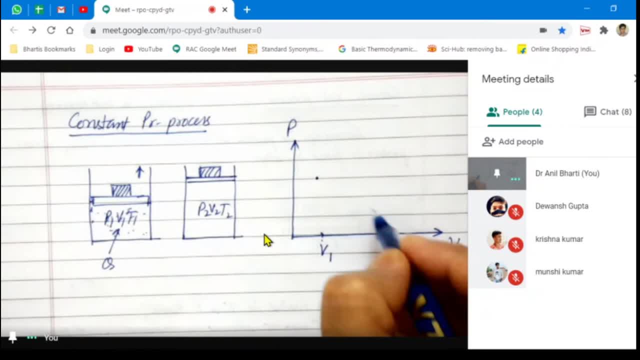 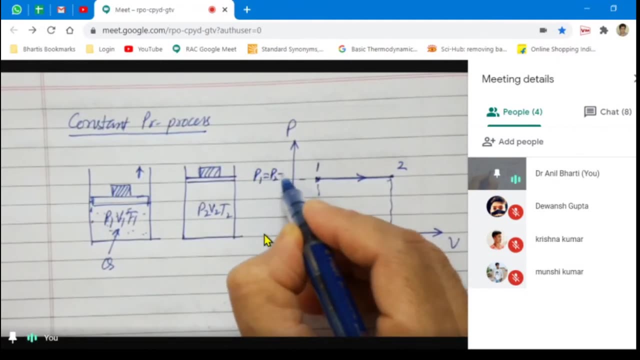 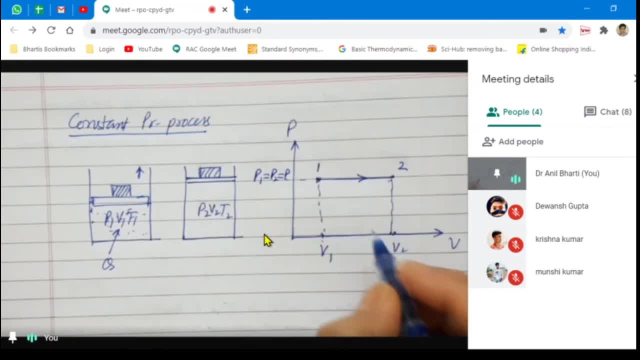 So you can easily find out the area under this graph, this line which is this, which is the shaded region, as I am showing here. So you can easily find out the area under this line and it returns to where at that Wu stop line is located. 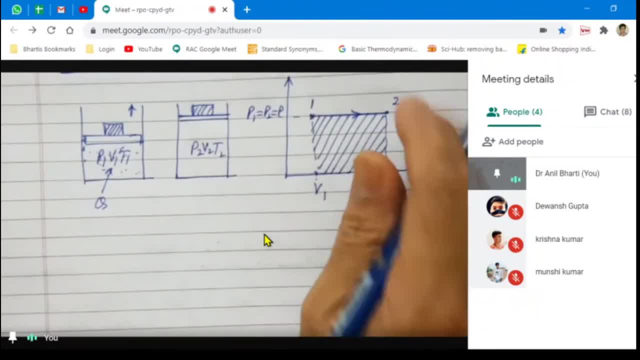 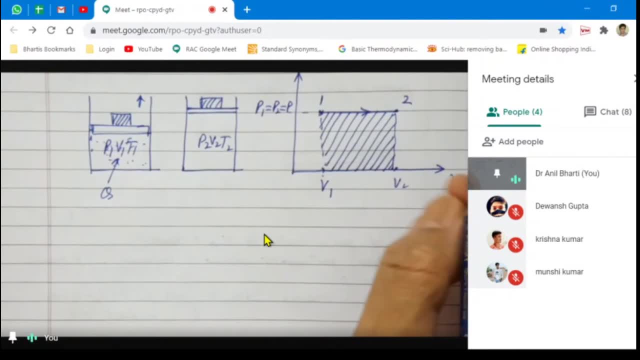 the this area. under this you can say shaded region. Now, if we can find out this area we can get the work done. So we can find. first we will find the work done for a constant pressure process. Now, work done is given by W is equal to 1 to 2 differential. this 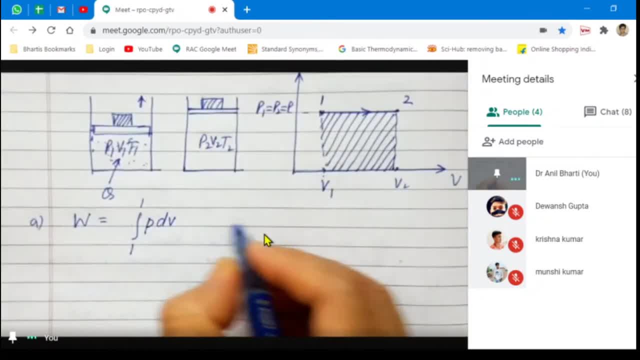 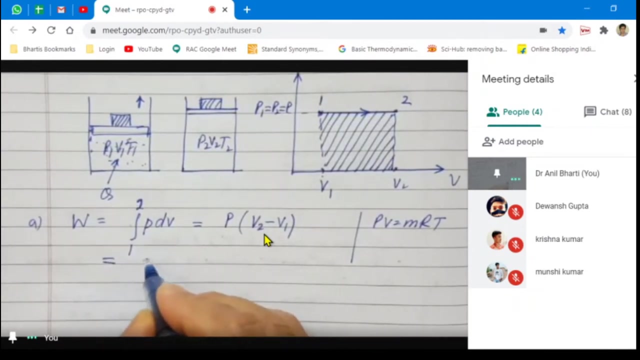 differential of P into dv, or this is equal to: since pressure is constant, P into V2 minus V1.. Now we also know this PV is equal to MRT, So we can also write it as: work done is equal to M into R, into T2 minus T1.. So this both. 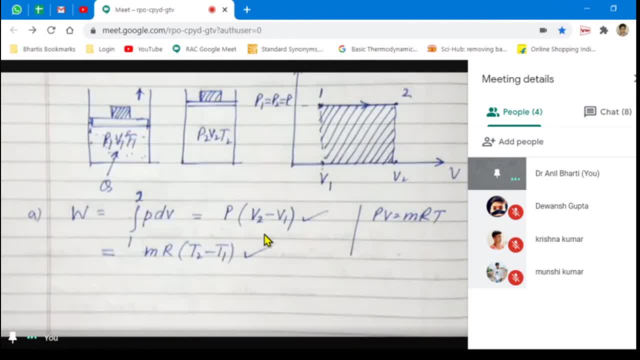 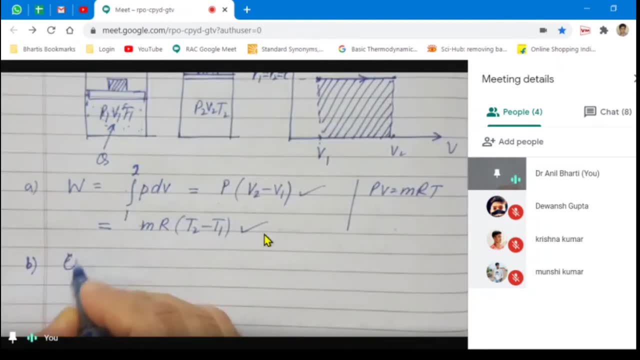 equations will chicken out we can use in this next section. second, is heat supplied? now, heat supplied Q is equal to this is a heat supplied into the system. now we know that whatever the heat is supplied, we can easily calculate it with the formula like mass of a gas into, since this is constant. 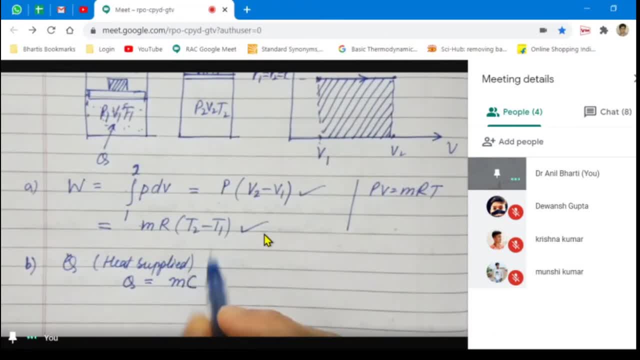 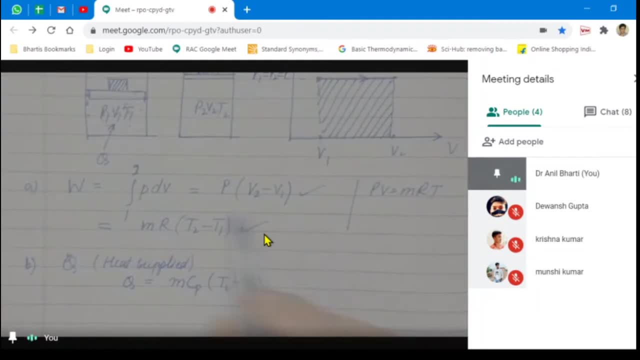 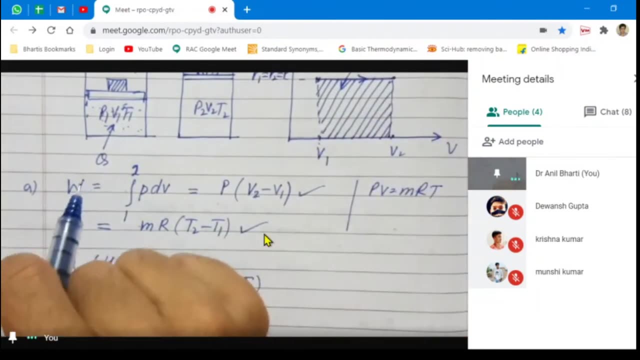 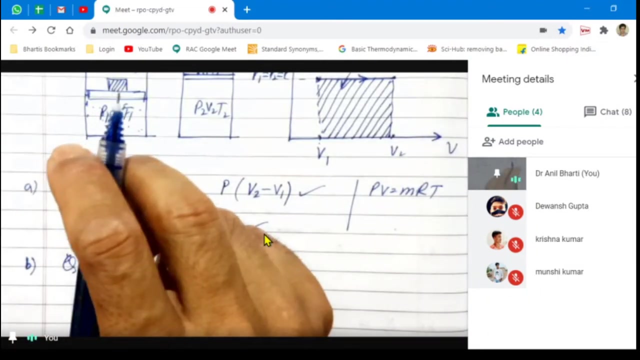 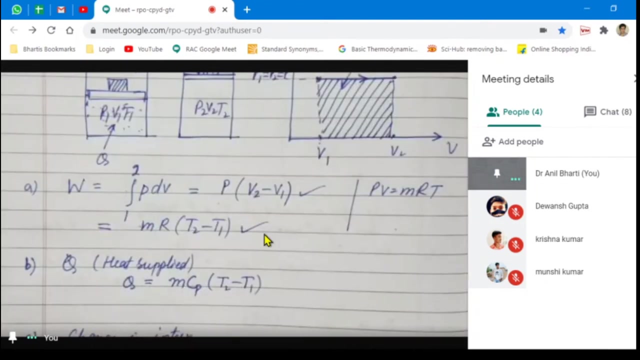 pressure process mass into Cp, into T2 minus T1 change in temperature. so this is the amount of heat transferred during the process. 1 to 2. so this is this much amount of heat is transferred into the system. so so. so similarly, in next we can find out the change in internal energy. 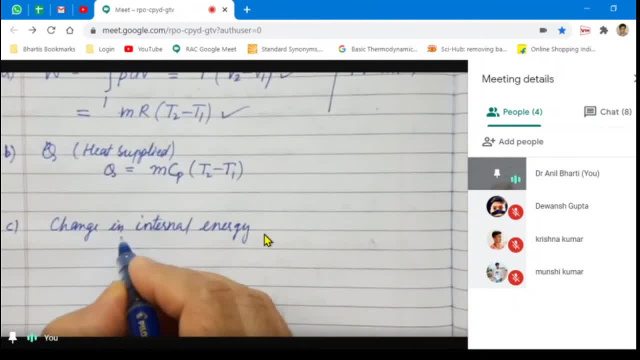 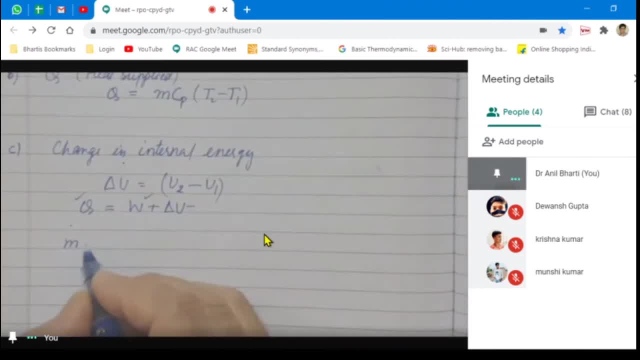 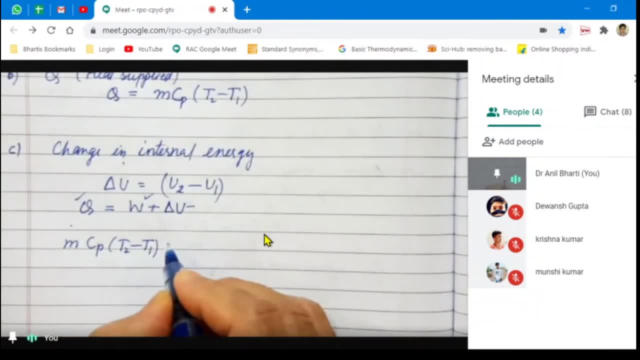 so so. so So W is M, R, T2 minus T1, M into R, T2 minus T1 and plus delta U. So from here we can say that delta U is equal to. you can also write down that delta U- change in internal energy is. 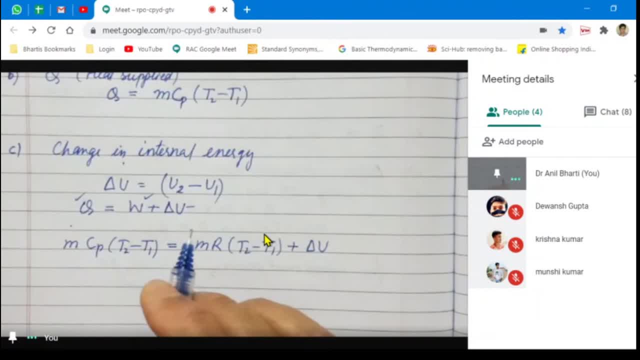 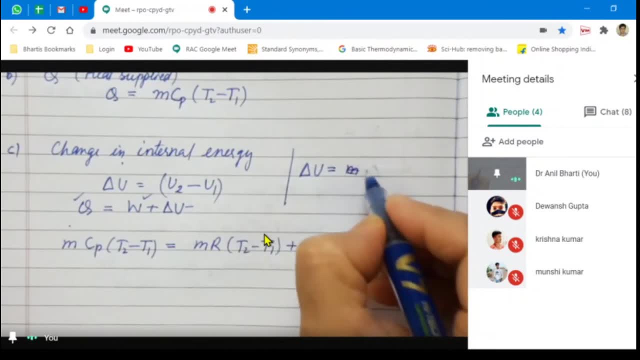 also having a unit of M- sorry M- into C, V, into T2 minus T1.. Internal energy: whenever you calculate it you should always write down that delta U is equal to. you can also write down that delta U, So again we can prejudice this equation. 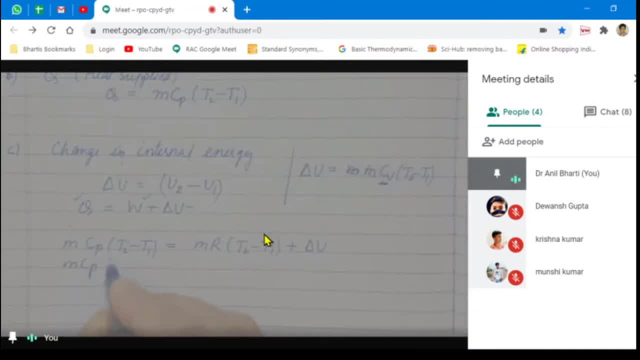 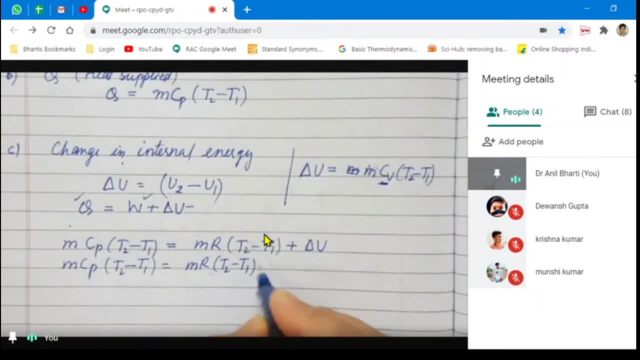 as M C, P 2 minus T1 is equal to M R, T2 minus T1 plus M. into C V 2 minus t1.. So, canceling out the common, this common terms we are left with- CP is equal to R plus. 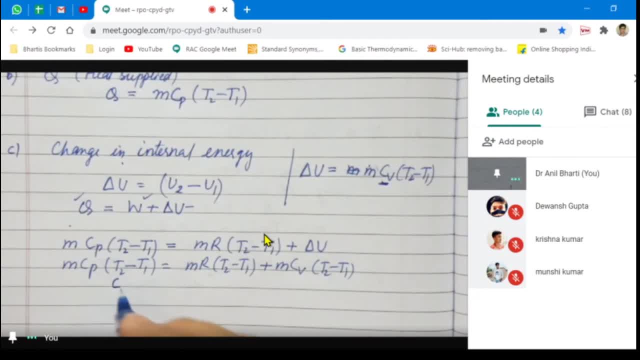 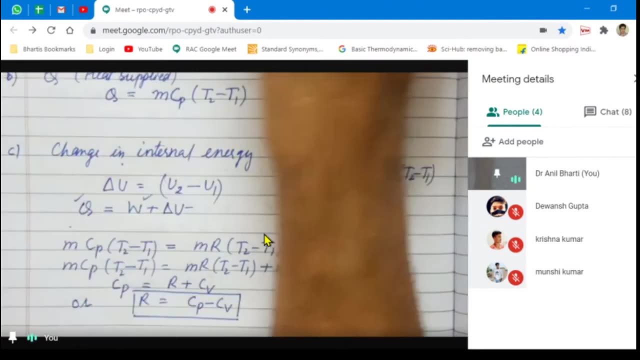 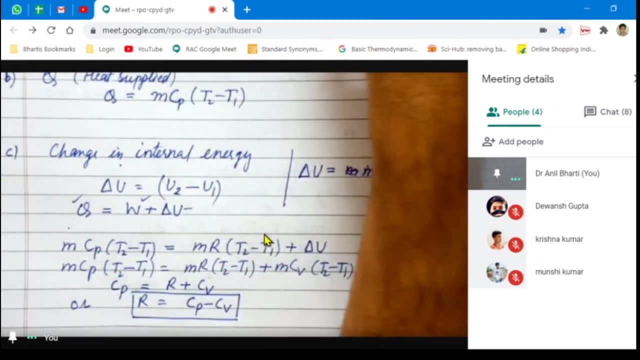 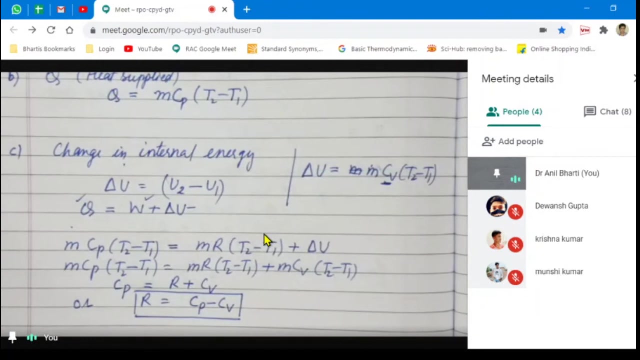 C, V. Okay, From here we get: r is equal to Cp minus Cv. You have already, I think, know this relationship, very important relation. So this is, you have this constant pressure process. This is also known as non flow process. Let's understand till here.